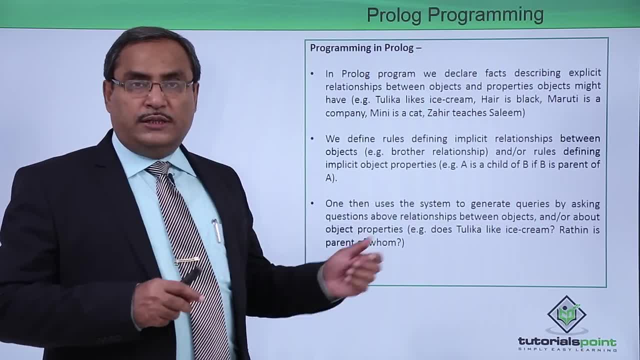 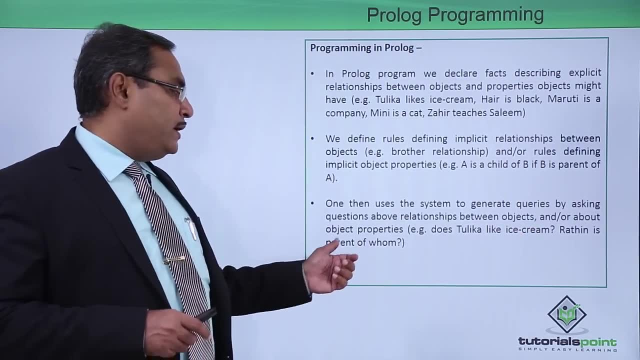 we are having some rules, So on those facts and rules, this query will get executed to give you the output, whether it is true or false. Rothin is parent of whom? So it will give you the answer: the respective child. So 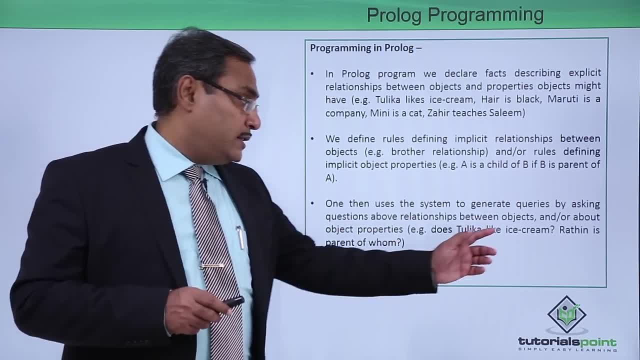 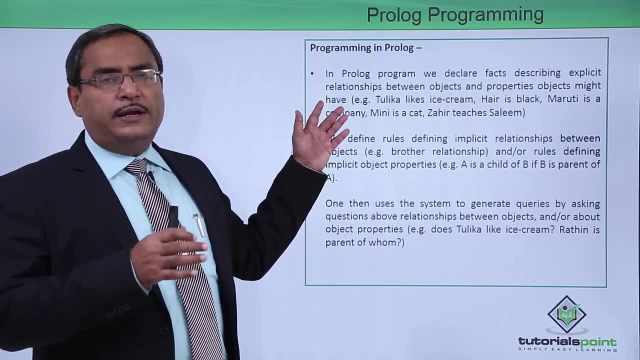 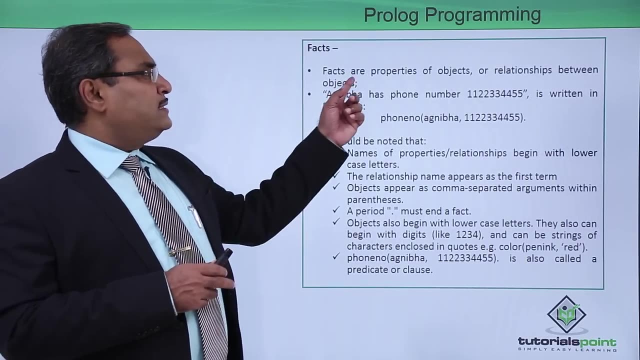 the child name of Rothin is if Rothin is really a parent of somebody. So in this way we have defined. to some extent we have defined our facts, rules and queries, So let us go for more elaborations. So facts are property, properties of objects or relationships. 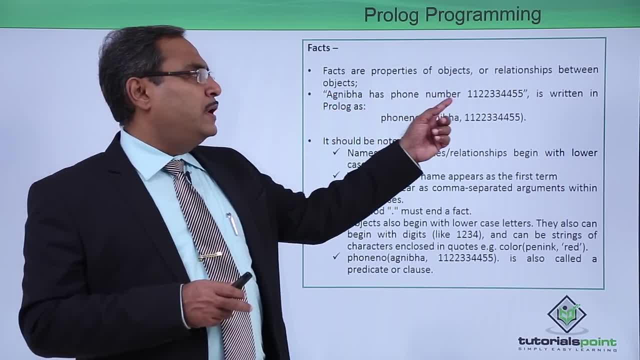 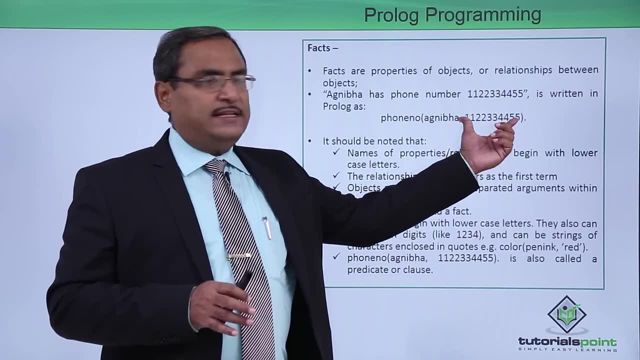 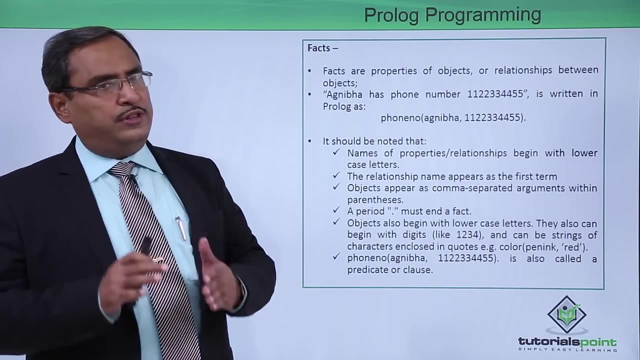 between objects. Ognevo has phone number. this is written in prologue as phone number or Ognivo and this, So in this way we can define that Ognivo is having the phone number that is 1, 1, 2, 2, 3, 3, 4, 4, 5, 5. in this way It should be noted that names of properties, relationships 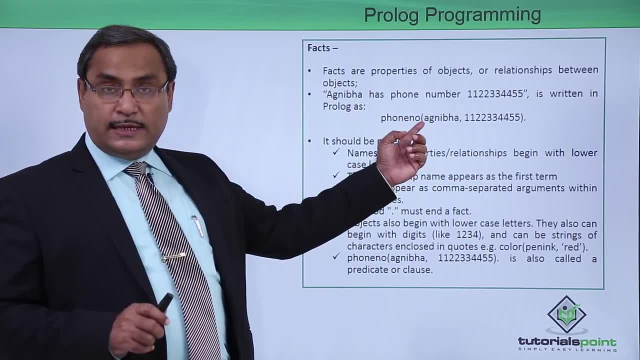 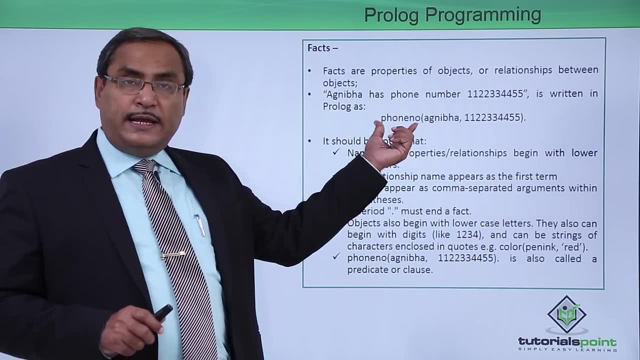 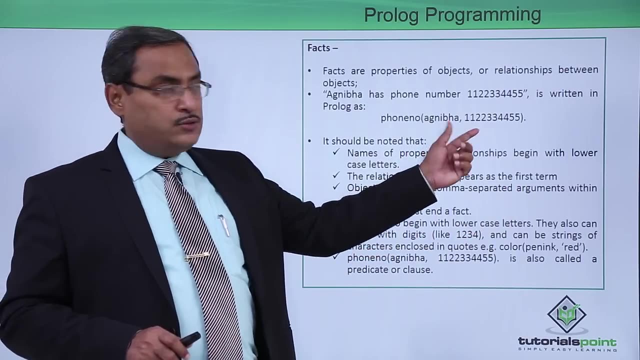 begin with the lowercase letter. So that is very important. The relationship name appears at the first term. The relationship name is appearing as the first term. Objects appear as commas, separated by arguments within parenthesis. So they will be separated by commas and they will. 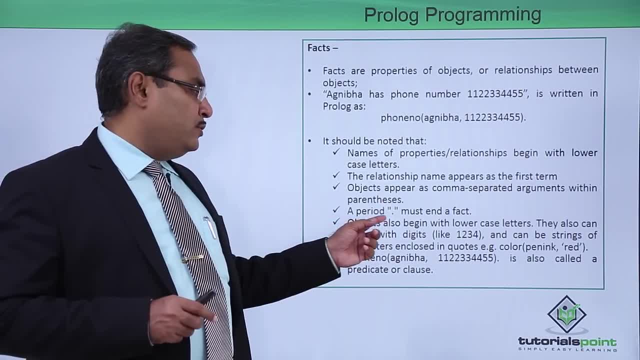 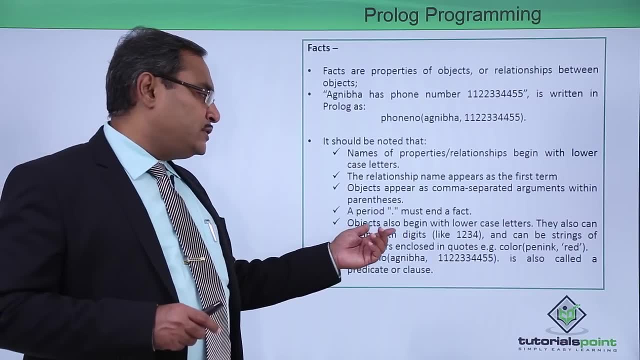 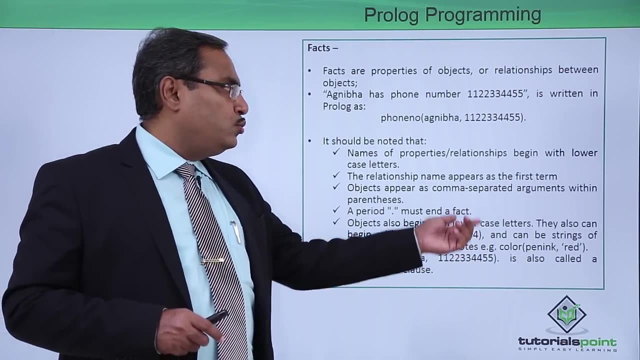 be kept within our parenthesis. A period must be there at the end of the fact, So period must be there at the end of the fact. Objects also begin with lowercase letters. They also can begin with digits, Like your 1, 2, 3, 4, something like this, and can be string of characters enclosed in codes As: 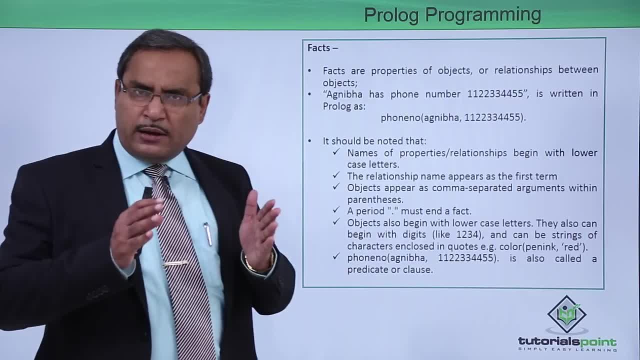 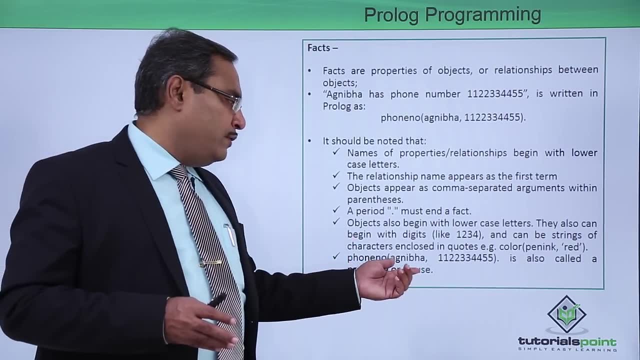 example color pink, red. So here we can write red without any codes, Otherwise we can put it in a code also. Phone number Ognivo 1, 2, 3, 4, 5, 5. 1 1, 2, 2, 3, 3, 4, 4, 5, 5 is also called a predicate. 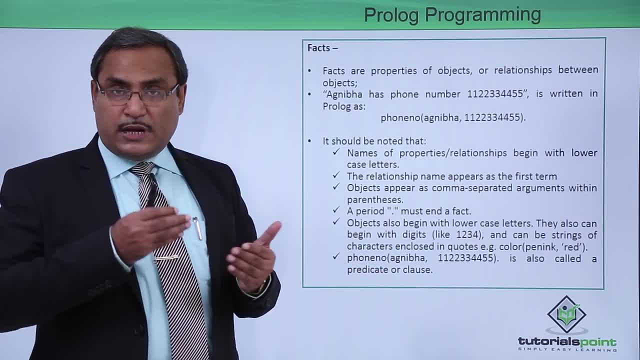 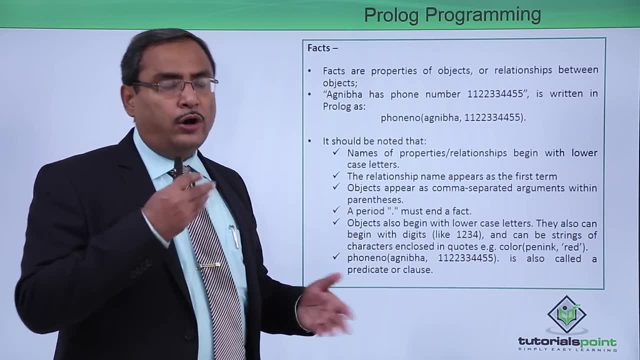 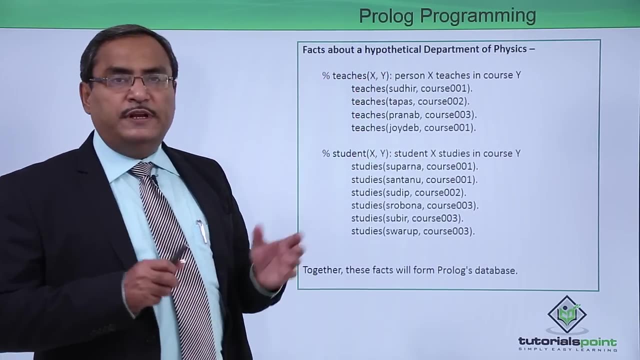 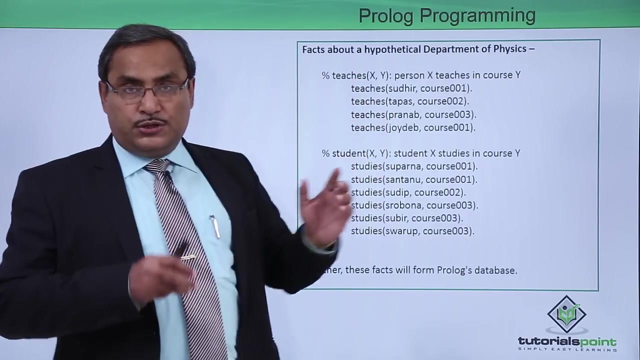 or a clause. So clause of same types will be known as a predicate. And clause can be divided. Either it will be of the type facts or it will be of the type rules. Facts about a hypothetical department of physics Teaches x y. Person x teaches in course y. So teaches x y means person x teaches in course y. 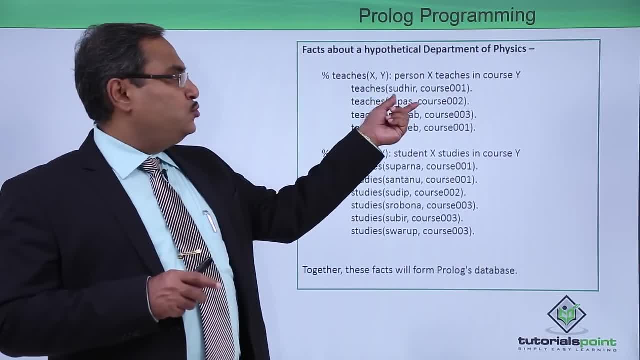 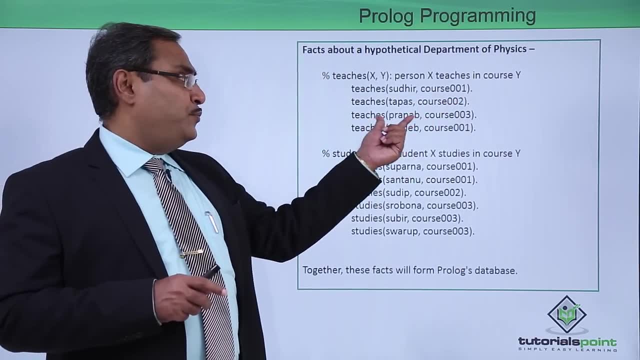 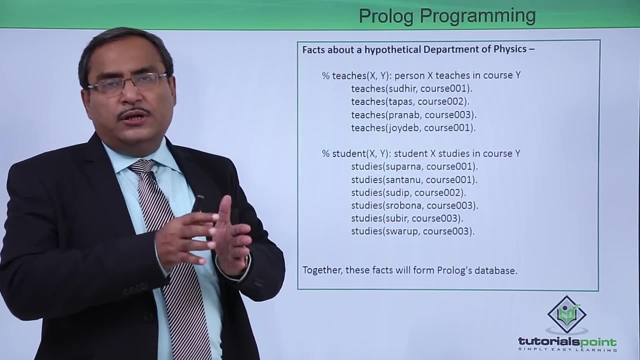 We are having this: teaches Teaches shudhir. This is the course id Taposh. This is the course id Teaches Pranav course id Teaches Jayadeep course id. So in this way we are having that who is teaching which course? And course will be denoted by the 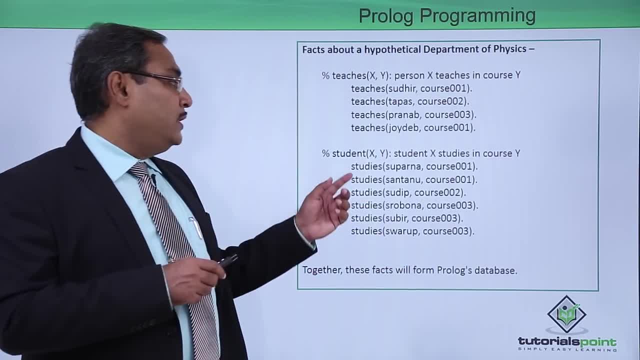 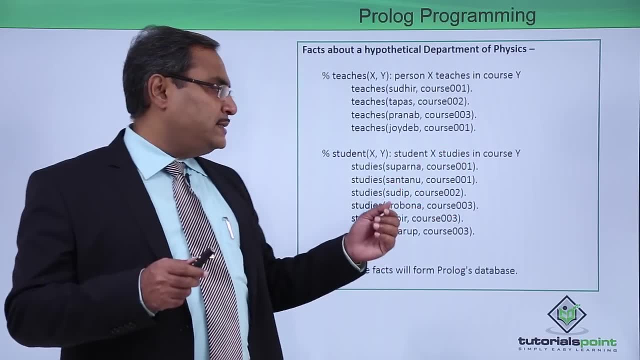 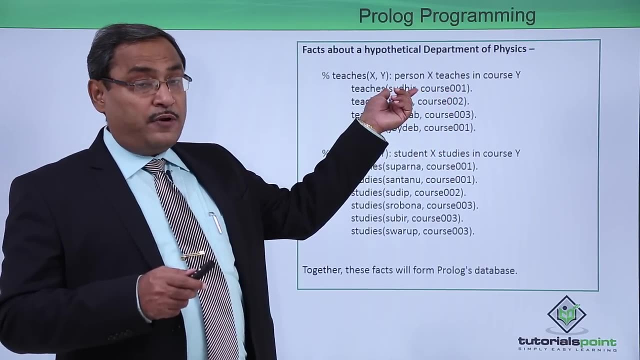 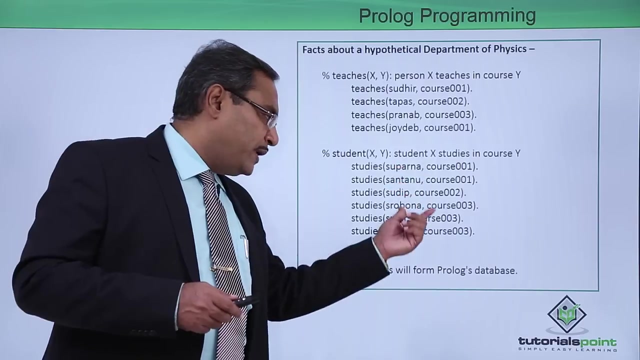 here in this example as course ids: Student x. y means student x studies in course y. Let us go for some example: Studies, suparna, course 001.. So that means where this shudhir was a professor. Studies. Shantanu quotes this: Studies Sudip quotes this. In this way we have 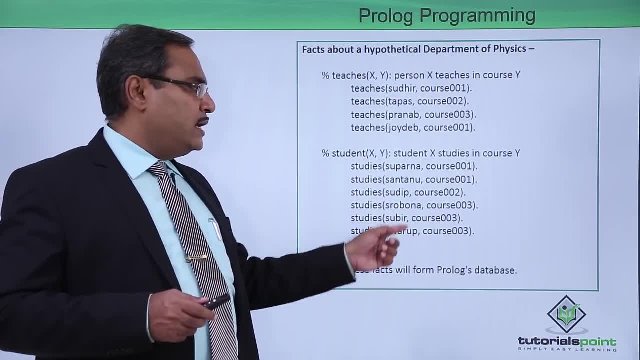 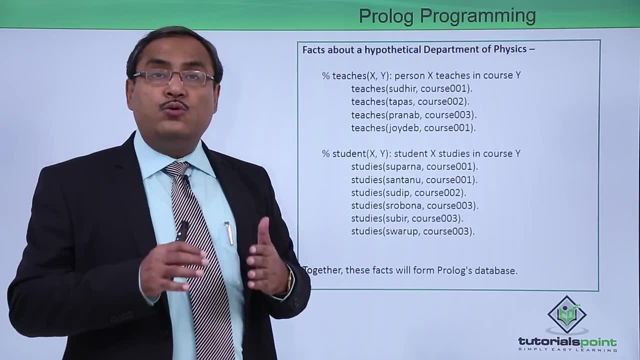 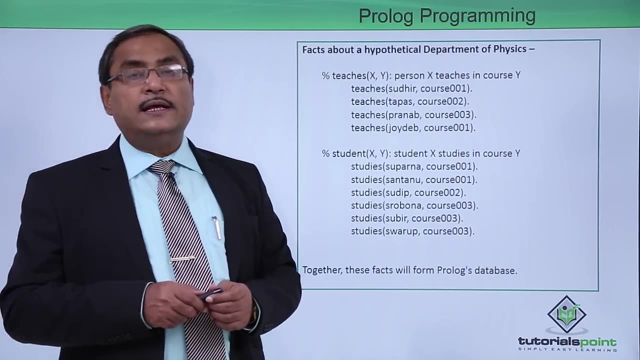 written. So in this way we have mentioned that who are the students and who is doing their study under which course. So in this way we have denoted that how to write facts there. Together these facts will form a prologues database, and sometimes it is also called as knowledge base. 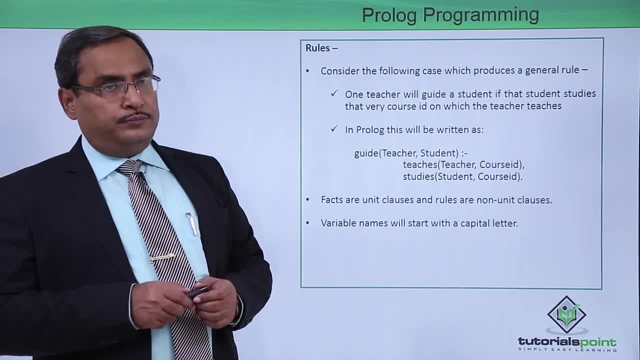 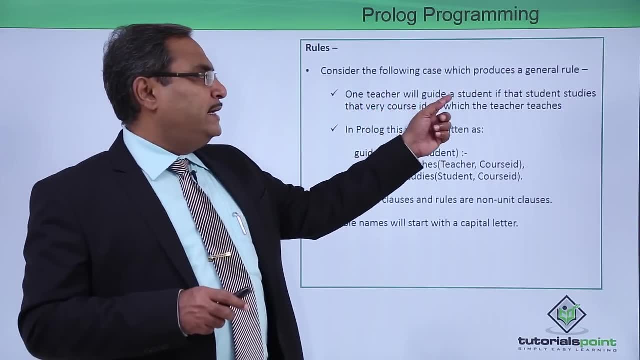 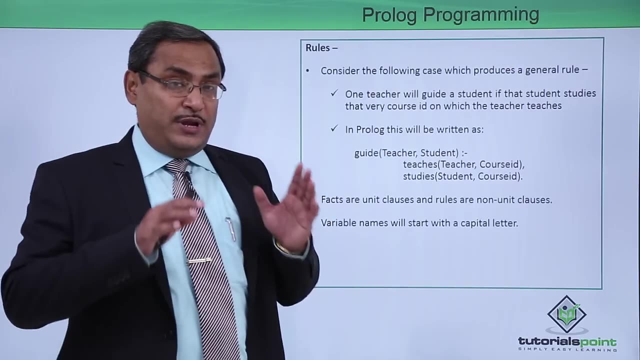 So now let us go for the rules. now Consider the following case, which produces a general rule: One teacher will guide a student if that student studies that very course id on which the teacher teaches. So if it is so, then we shall say that we are forming one rule In prologue. this will: 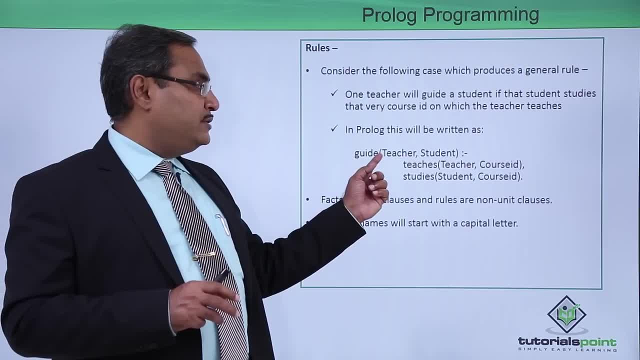 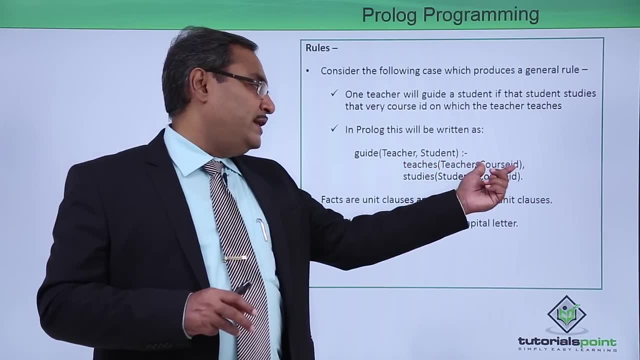 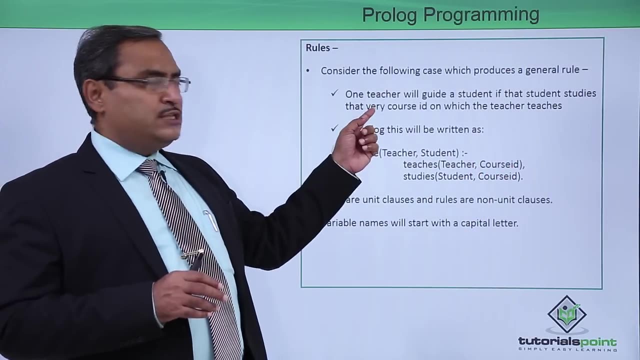 be written as guide teacher. Here you see, the first letter is capital, So it is a variable. So teacher, teacher, student teaches teacher course id and studies this student same course id. So in this way this rule, which was written in plain English, can be formulated in the prologue. 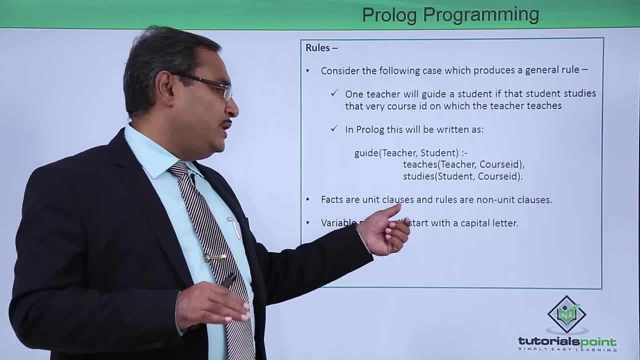 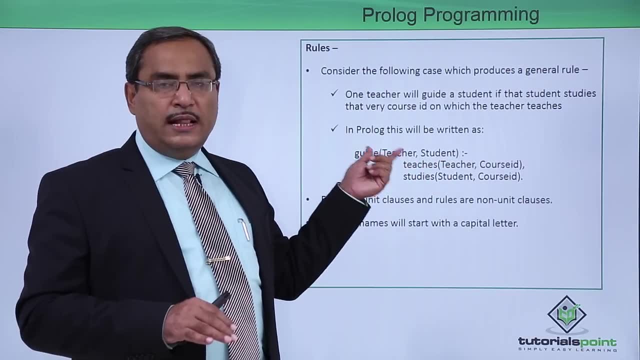 clauses in the form of rules. Facts are unit clauses and rules are non-unit clauses, because here in case of rules we are having multiple components, are there left hand side, right hand side- in this way, So here it can be expressed in multiple clauses, also Variable. 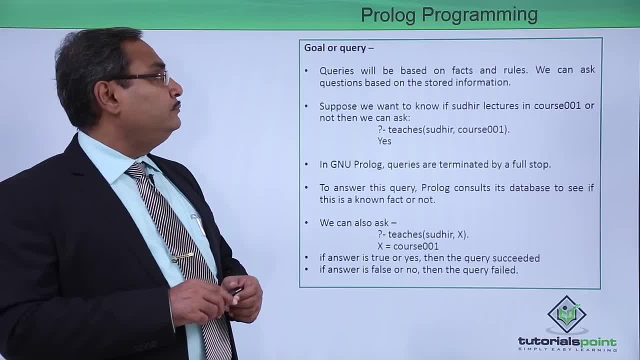 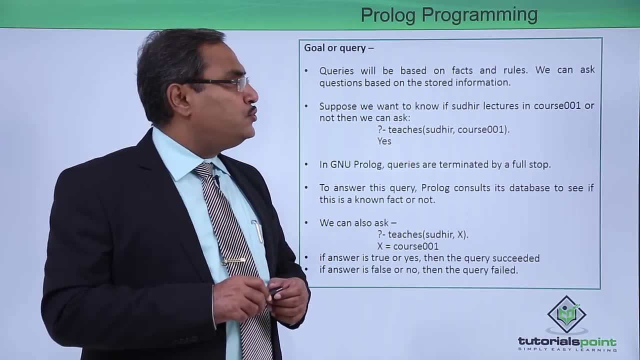 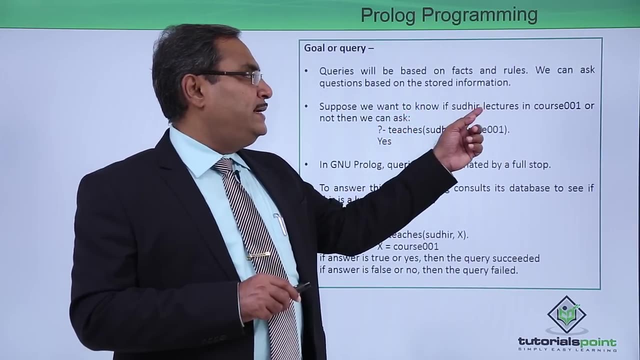 names will start with a capital letter. So now let us discuss this goal or query. Queries will be based on facts and rules. We can ask questions based on the stored information. Suppose we want to know if Sudhir lectures in course 001 or not, then we can ask teaches. 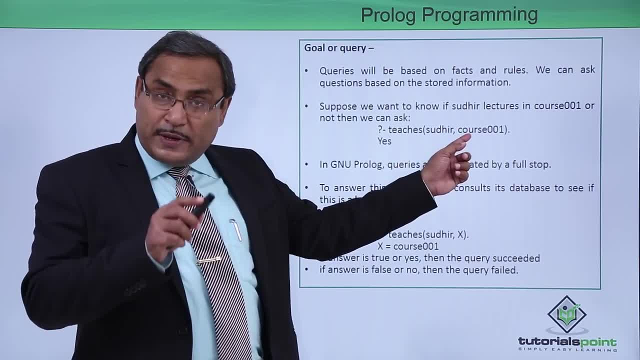 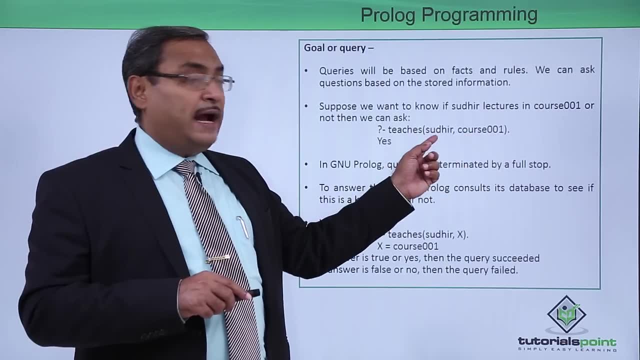 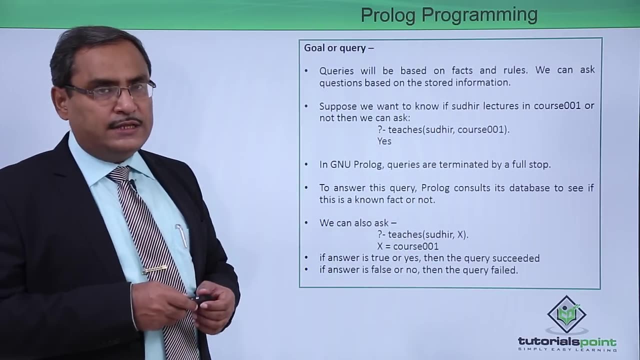 Sudhir In course 001, then the respective facts will be checked and here in our knowledge base, in our database, whatever we have discussed, this fact is existing. So the answer will be coming as yes. but for other combination it might be coming answer as no or fail. 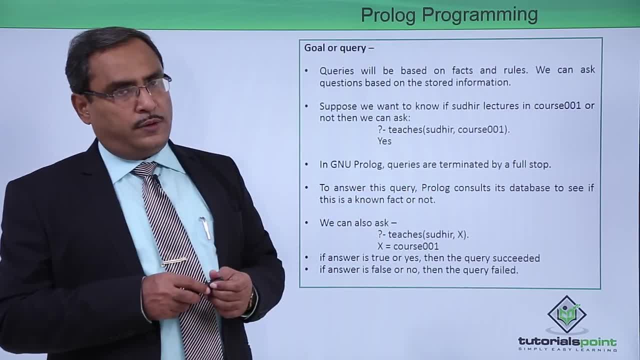 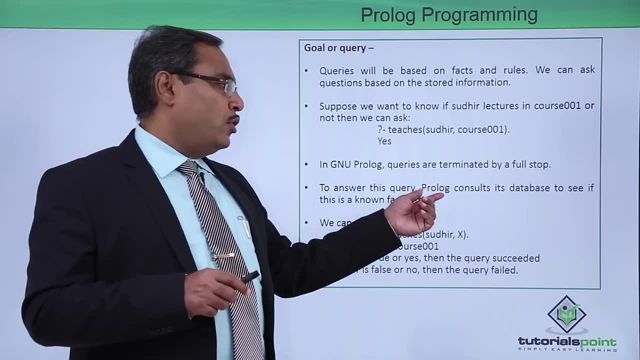 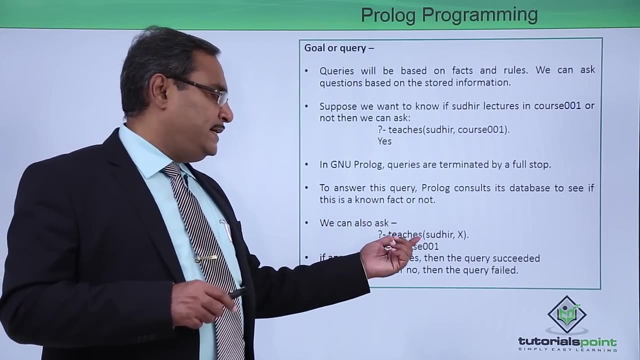 In GNU prologue queries are terminated by a full stop, So in GNU prologue we will be terminating each and every query by a full stop. To answer this query, prologue concept says its database to see if this is a known fact or not. We can also ask: teaches Sudhir? 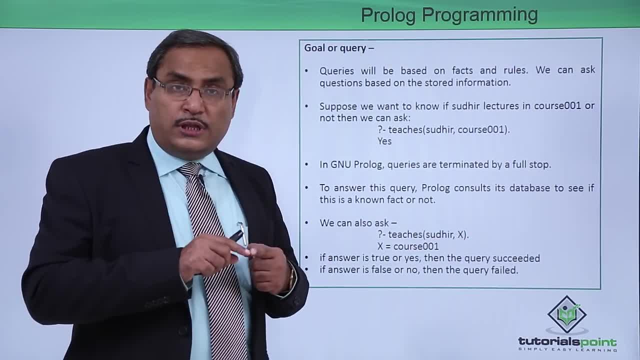 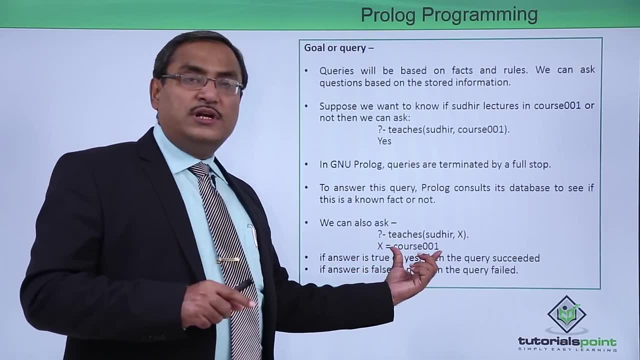 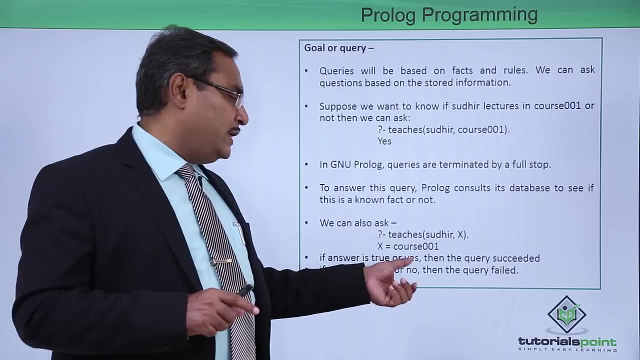 x. X means a variable, So I want to know the Sudhir this professor teaches. in which course In that case, x will be coming, as, say, course 001, because it was mentioned in the knowledge base in the form of facts. If answer is true or yes, then the query succeeded. 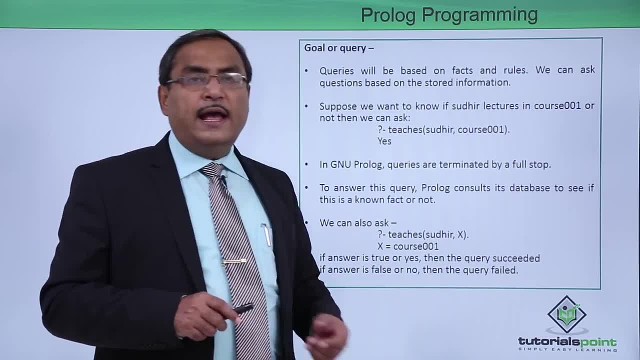 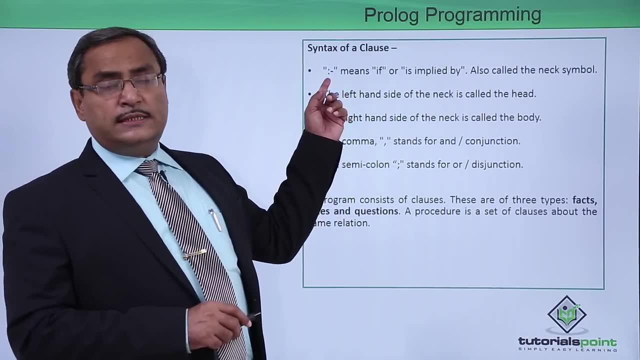 If the answer is false or no, then it cannot be proved. So the answer is也. So I am going to subscribe to my channel and I will see you in the next lecture. then the query has failed. Let us discuss syntax of a clause. So this colon dash means if or is. 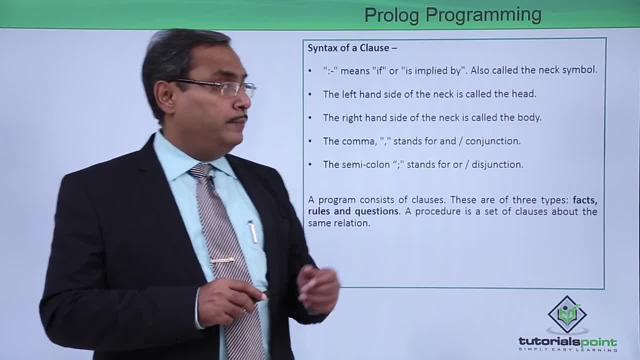 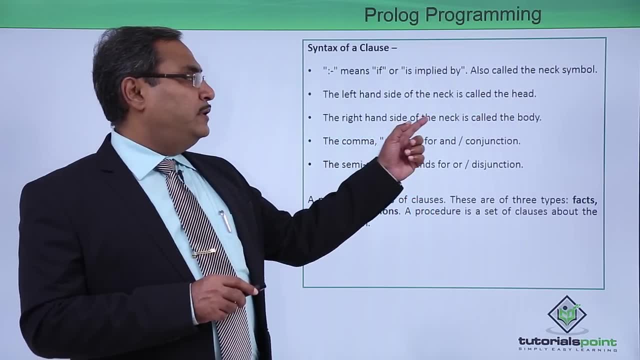 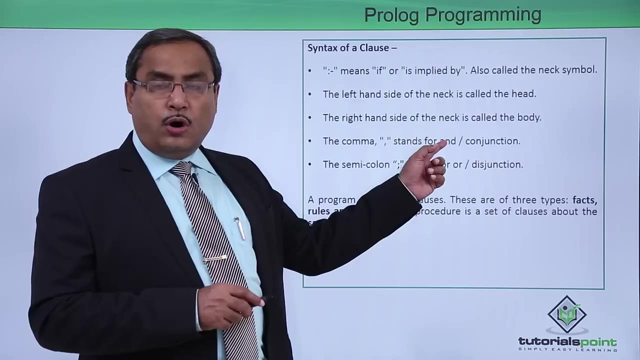 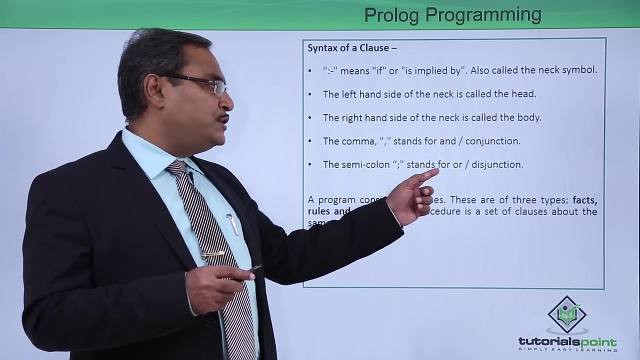 implied by also called the neck symbol. The left hand side of the neck is called the head, The right hand side of the neck is called the body. The comma stands for, and or conjunction. The semicolon, if we put semicolon in place of comma, stands for, or or disjunction, A program. 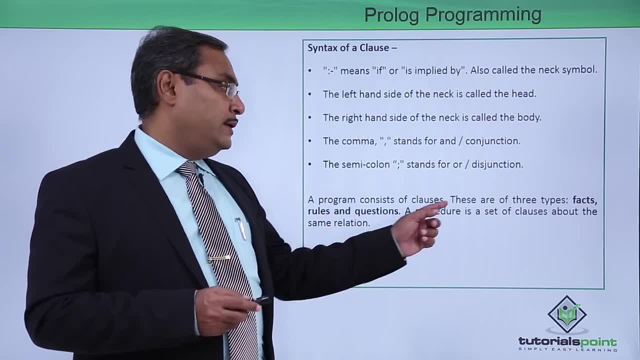 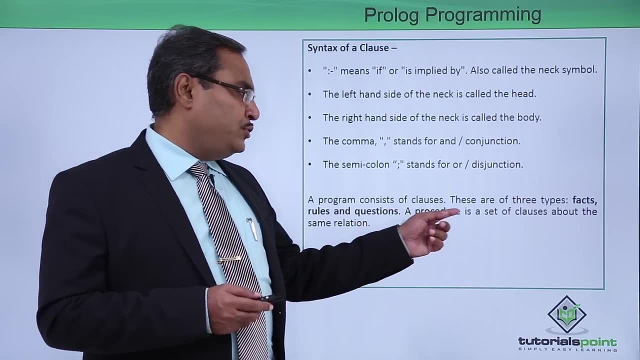 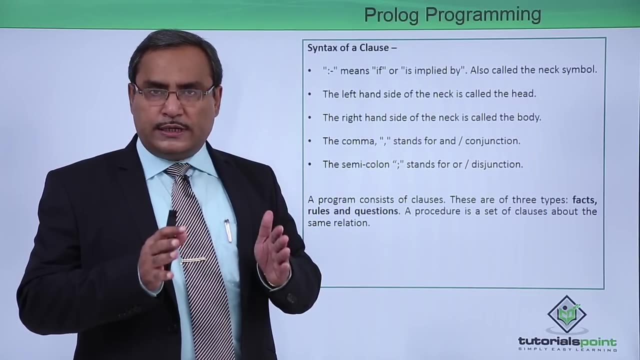 consists of clauses. We discussed this one earlier. These are of three types: facts, rules and questions or queries. A procedure is a set of clauses about the same relation, So a procedure is a set of clauses about the same relation, So that is known as the procedure. So we are having 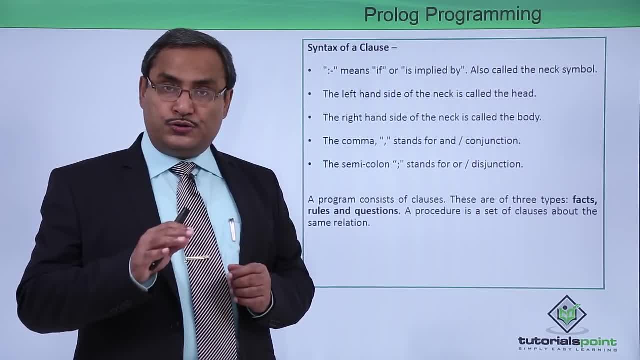 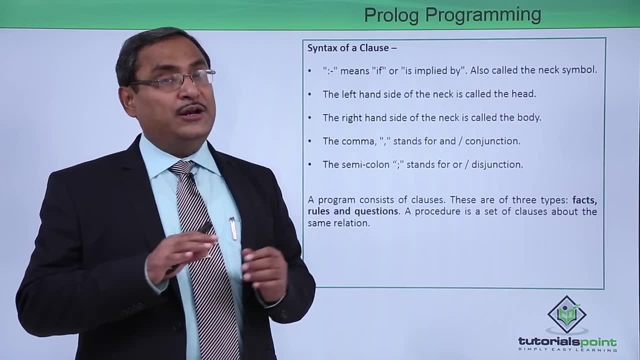 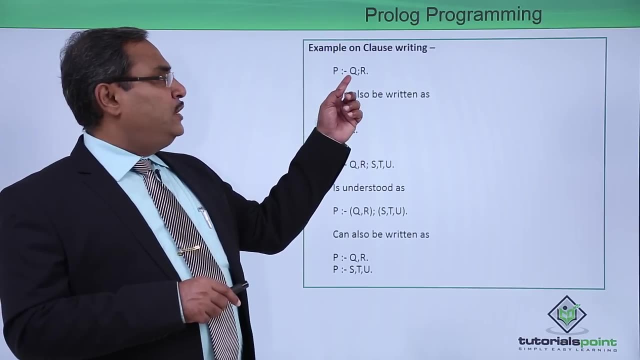 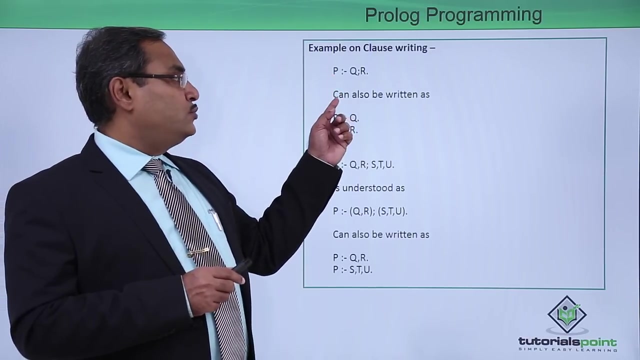 different terminologies, So facts, rules, queries or questions. we are having here procedures, clauses, predicates and so on. So example on clause writing P is a person who has one if q or r. q and r both are written in capital letters like p, so they, all of them are variables. 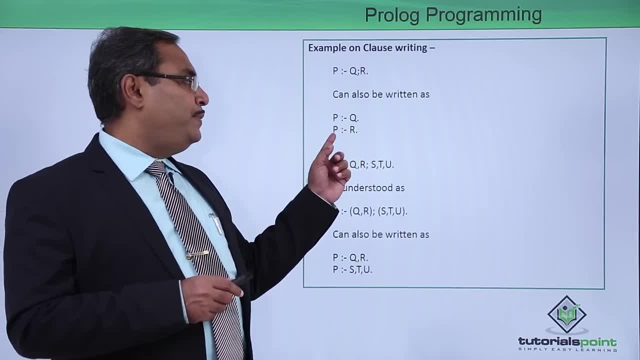 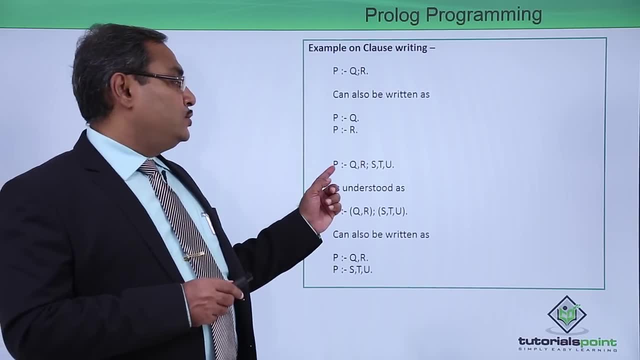 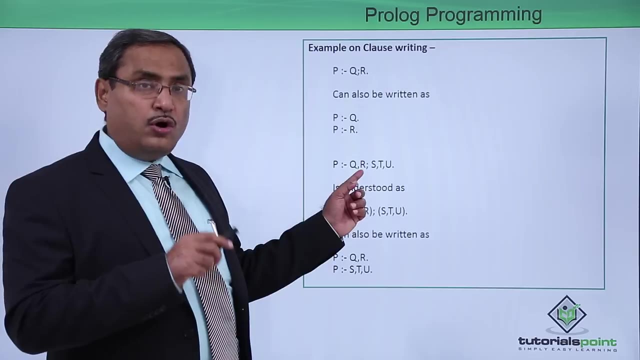 so can also be written as p if q, p if r, because here they are connected by or logic, so or means disjunction, So p q, r, that is, and p if q and r, or semicolon s and t. 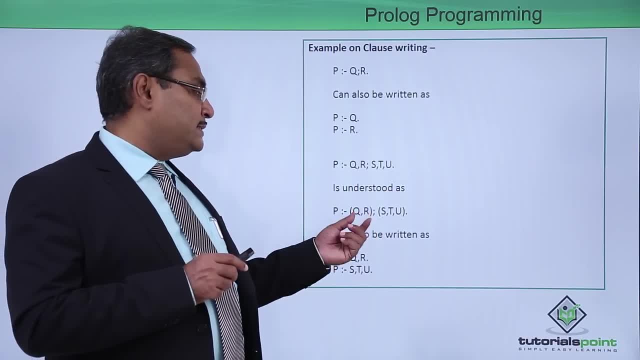 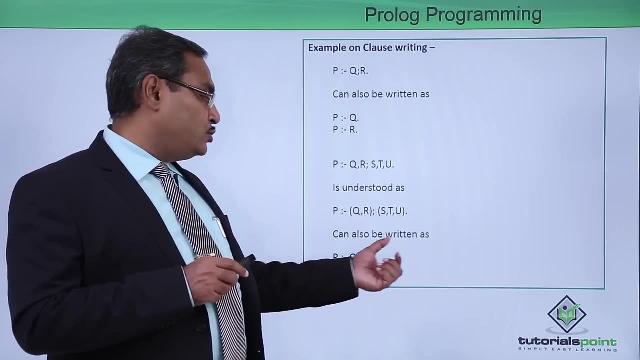 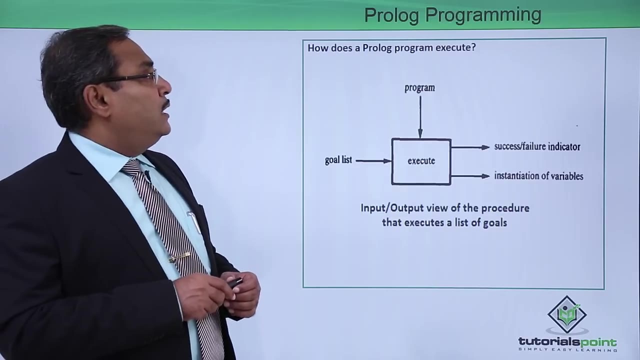 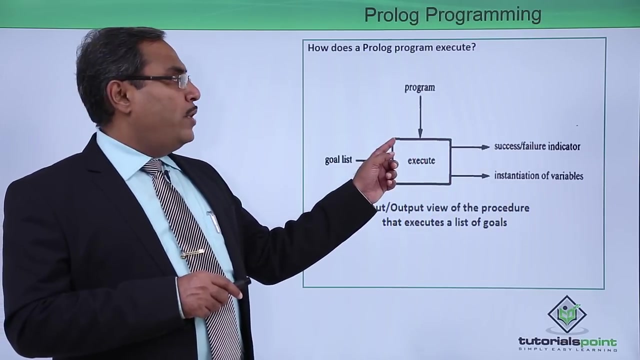 and u, full stop is understood as p, q and r or s and t and u can also be written as in this way. So in this way we can write our rules. How does a prologue program execute? So this is: execution is taking place, we are having the program taking the program. 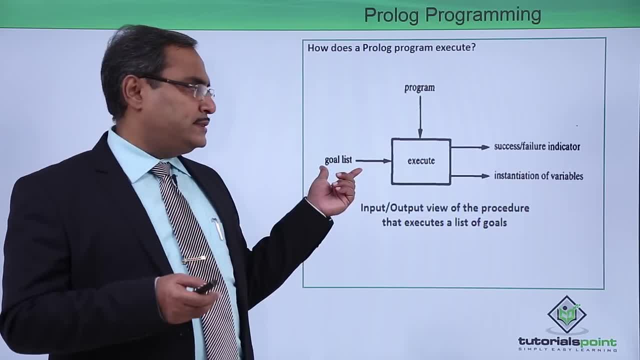 as input. we are having some goal list, some queries or questions. So we are having the program as input, we are having some goal list, some questions. then outputs will be coming in the form of Boolean that is success or failure. 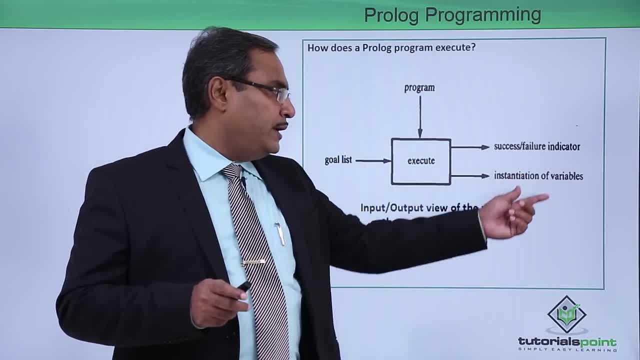 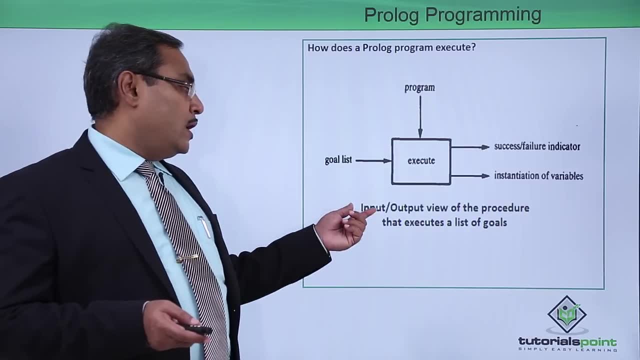 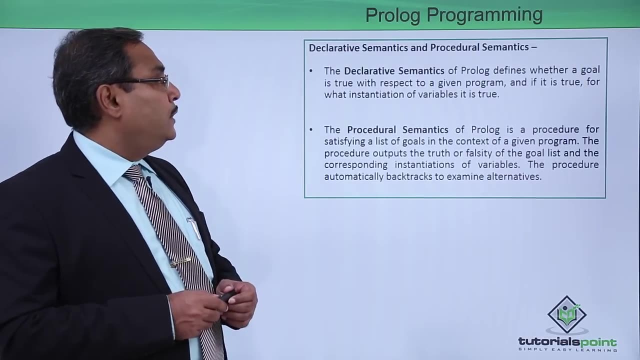 yes or no, true or false or fail in this way. Otherwise it will instantiate one variable, so in this way the outputs can be obtained. Input-output- view of the procedure that executes a list of goals. So now let us discuss decorative semantics and procedural semantics. 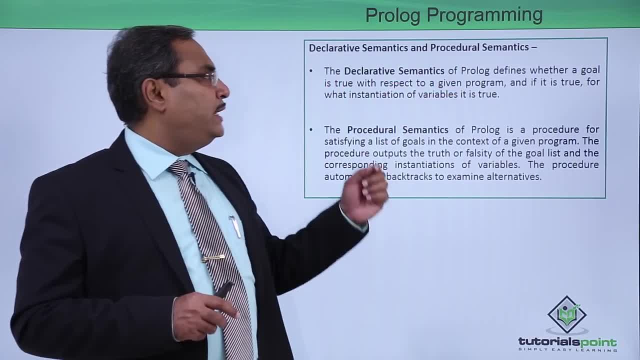 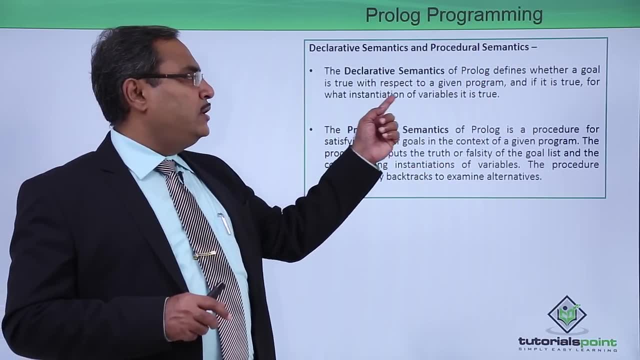 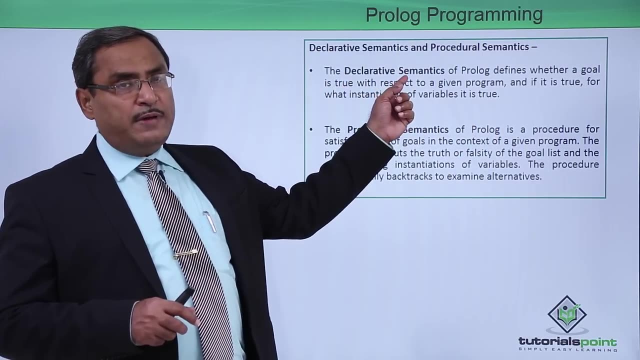 The decorative semantics of prologue defines whether a goal is true with respect to a given program and, if it is true, for that instantiation of the variables. if it is true in that case, That means it is telling that in case of decorative semantics depending upon the given program,